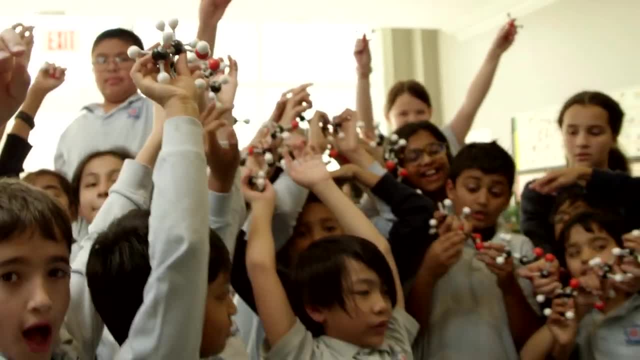 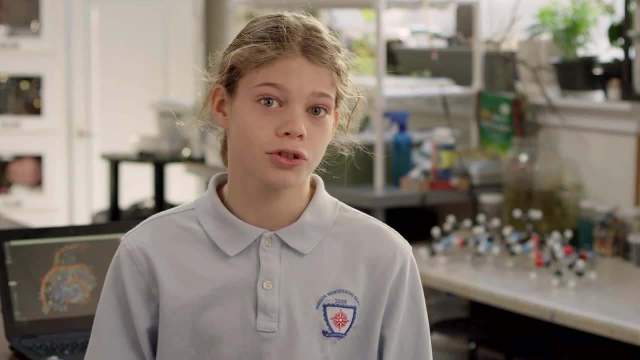 People have access to. I really think that everyone from a very early age should get this and should feel confident and comfortable with it and be able to connect to this amazing high-tech society that we live in. I usually never get anything like this in school and I like science and technology. 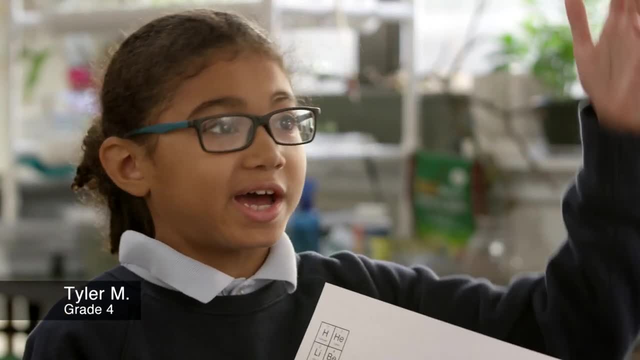 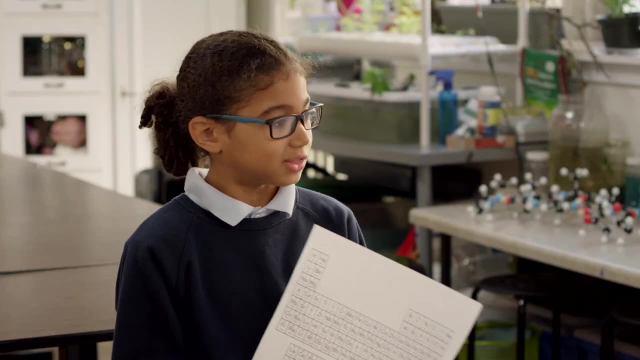 I just thought, oh, this is like the ground and this is the sky. But now that I know biochemistry, I can like tell like what atoms are in what? like the ground, the sky, the walls, Like if there's iron in the walls or there's metal in the walls. 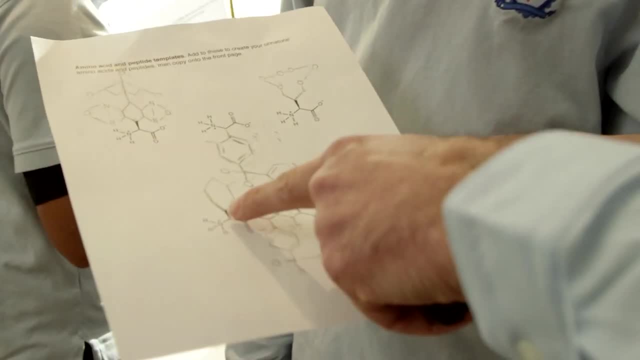 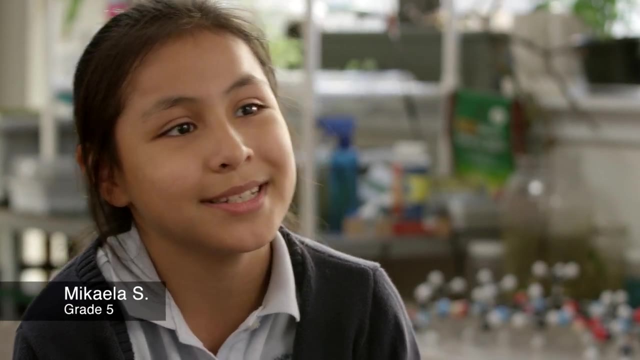 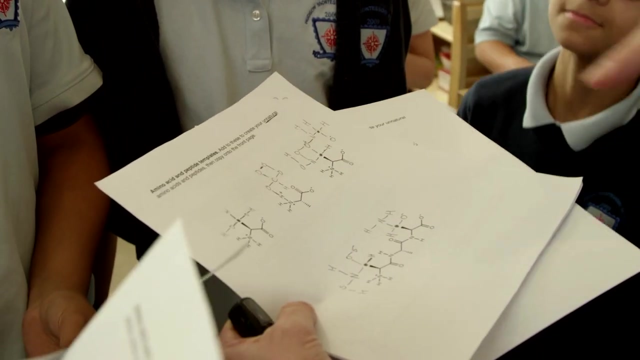 We get to learn about atoms, molecules, and we go really in-depth about it. I learned about a mole like not the mole that digs in the ground, but if it was a carbon mole or oxygen mole or a neon mole and they'd have a certain amount in each one. 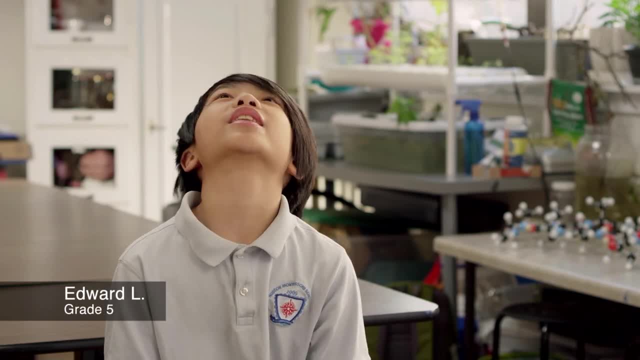 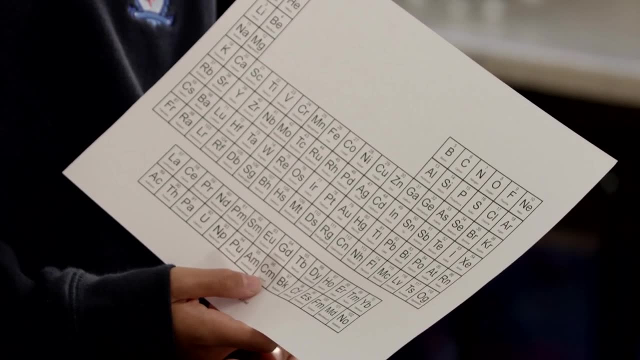 I really liked it, And like because the fact that we're at the same levels, like people who are much older than us. The octet rule is when an element has two electrons in the first orbital and eight electrons in the second orbital. 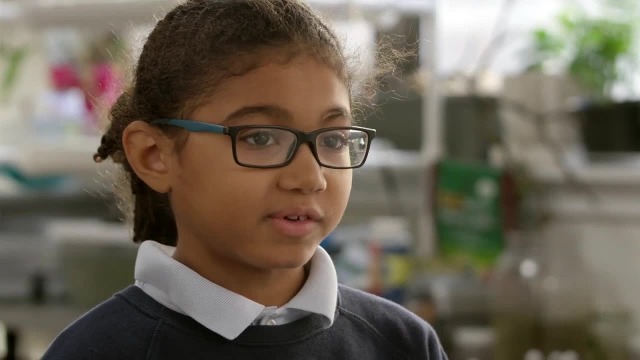 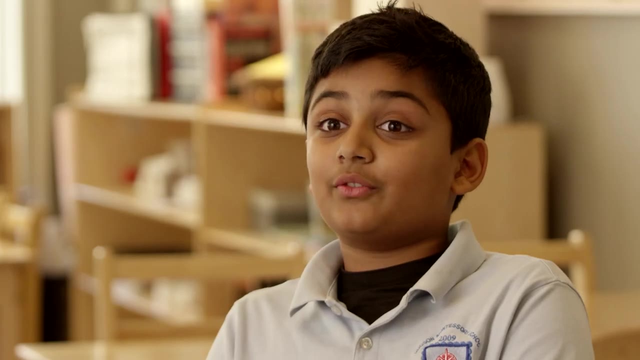 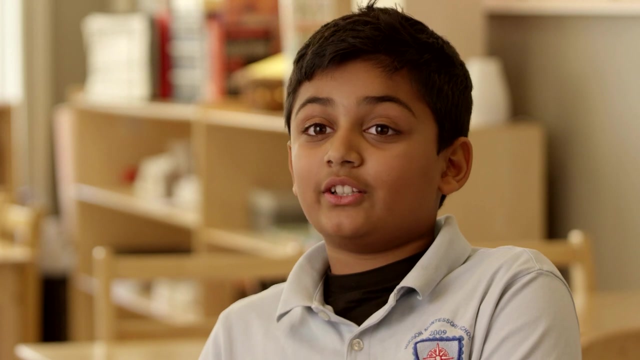 That's what we call an octet. Since neon doesn't have any bonds left, then all the electrons are happy and they can't bond with any other elements. I think it's really joyful to know you're knowing a college education, because I didn't know I could achieve all the information. 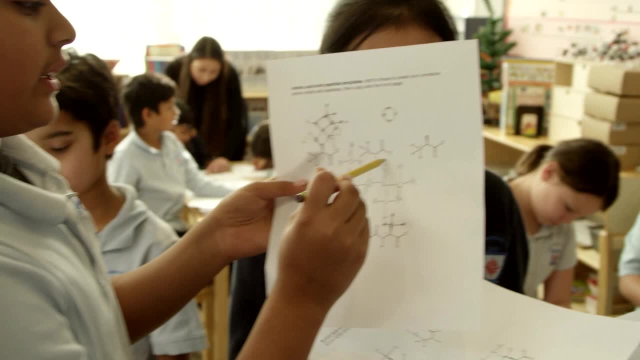 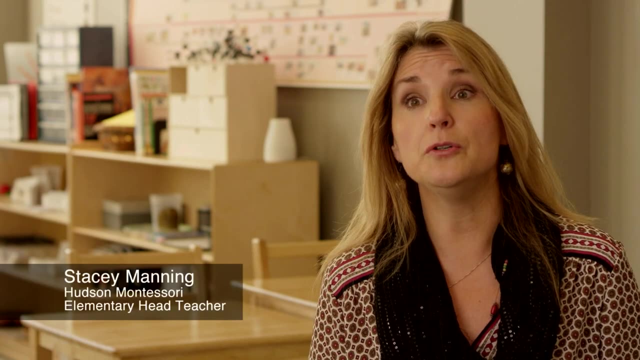 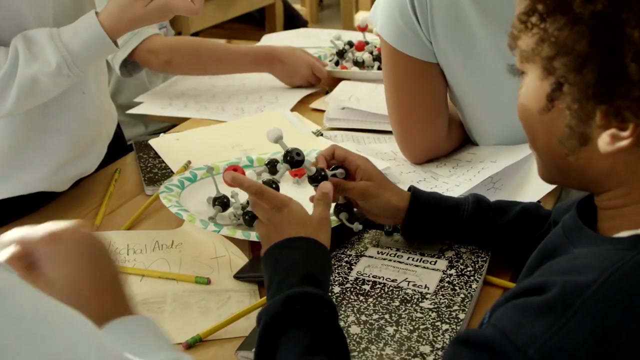 I've learned from molecules to pi-moles to DNA. So the approach that Dr Fried is taking with this program really allows the children to use all of their learning skills. He uses hands-on materials, he gives visual presentations and then he lets them apply their knowledge. 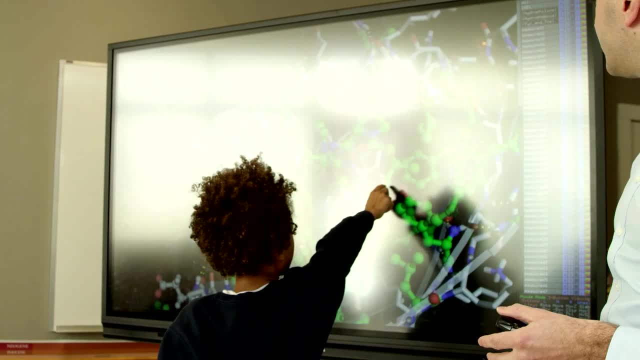 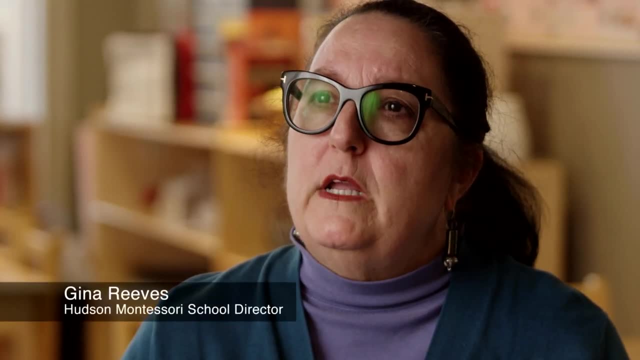 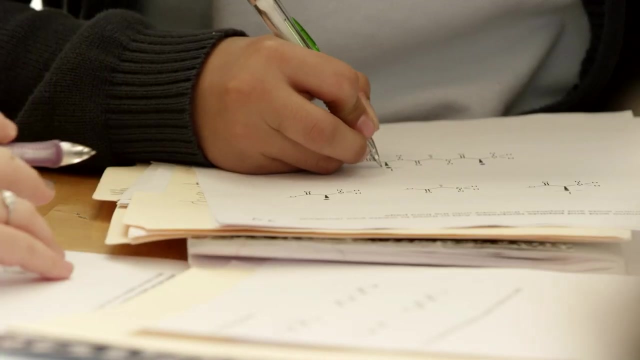 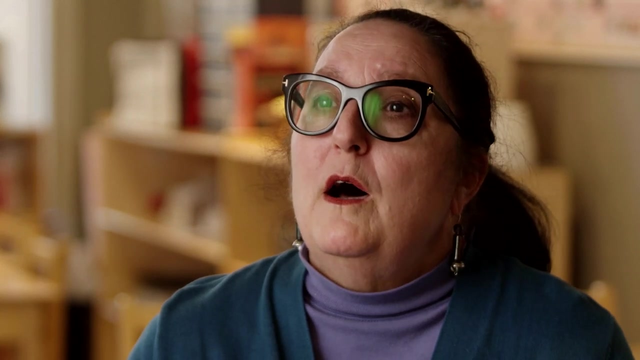 And this has really made the kids enthusiastic and excited, Excited about this program. You bring in the hands-on and you bring in the pictorial so that they could really understand and break into bite-sized pieces and gain a greater understanding. They're excited about what you're doing, they're excited about the learning and that kind of excitement is what engenders a passion. 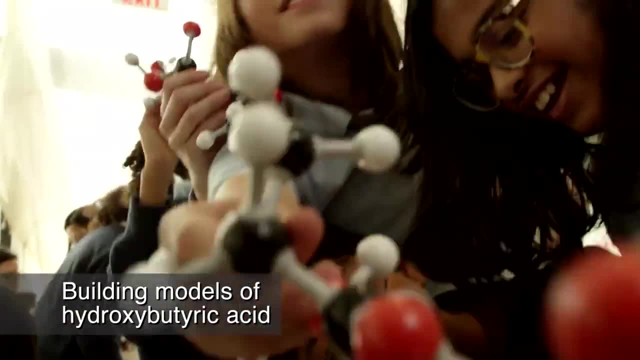 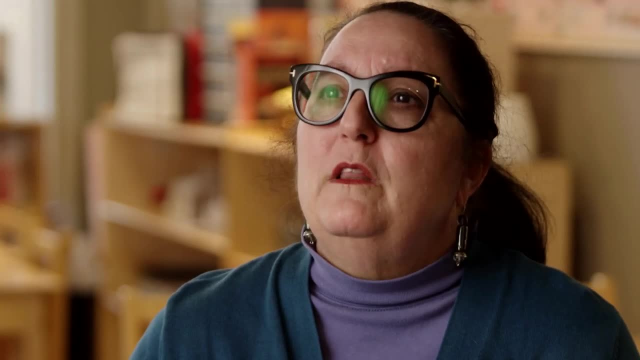 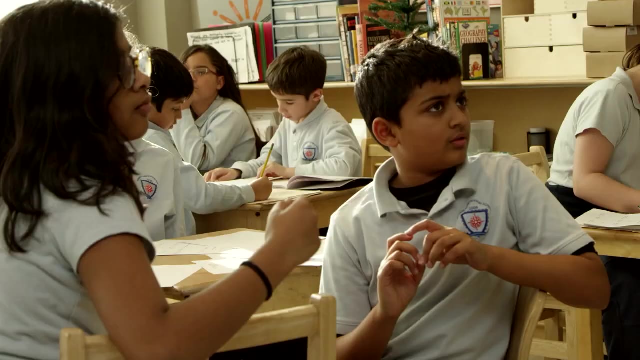 So you can hear them in the hallway talking about science and talking about biochemistry and talking about the different things that they have made And that's really true, wondrous learning. They talk about it all the time They go home. The parents are coming to us telling us what their kids are saying and how they're expressing their love of biochemistry. 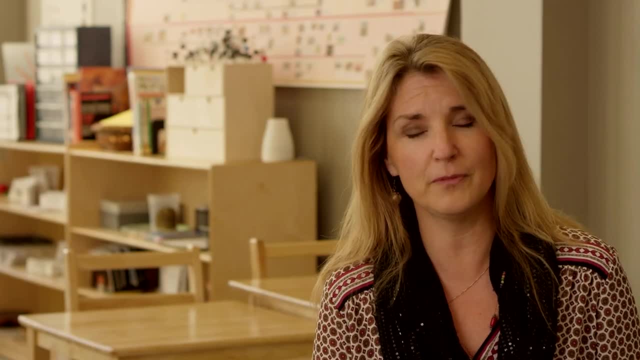 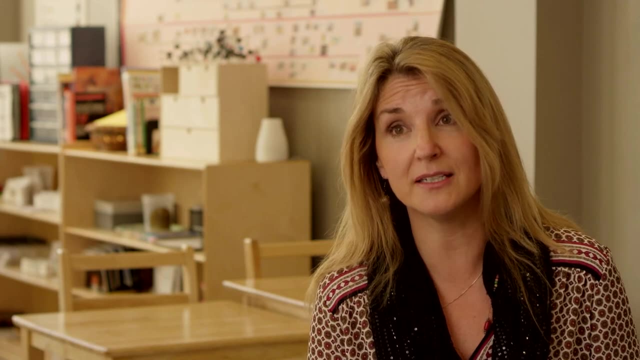 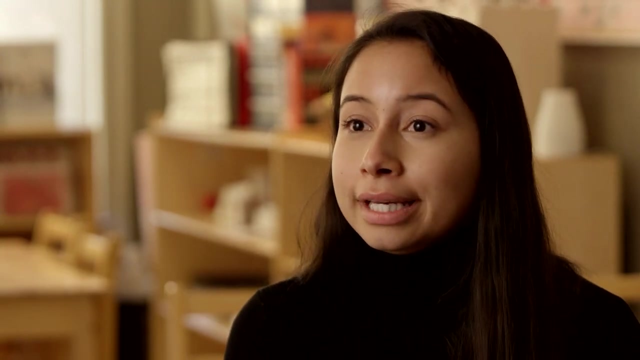 And they can't believe it. The parents are absolutely floored that their children not only are learning this, but understand it. As somebody who took biochemistry- and wanted to- in college, I was really fascinated. I was really fascinated and impressed by how quickly and easily these kids were able to understand these concepts. 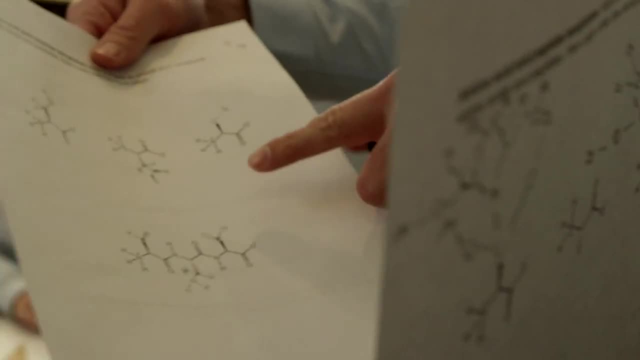 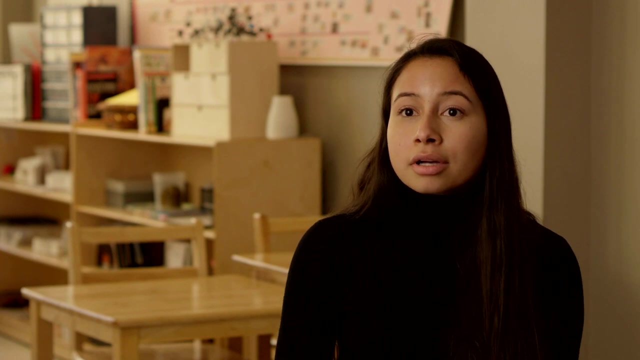 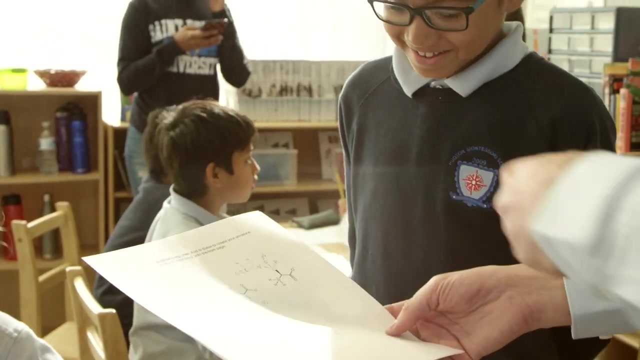 And not only that, how quickly they understood the relationships between physical and biological function, as well as theoretical and empirical concepts, And it was really impressive to see how they made these connections with only a few classes And, in comparison, it took me and, I'm sure, most college students. 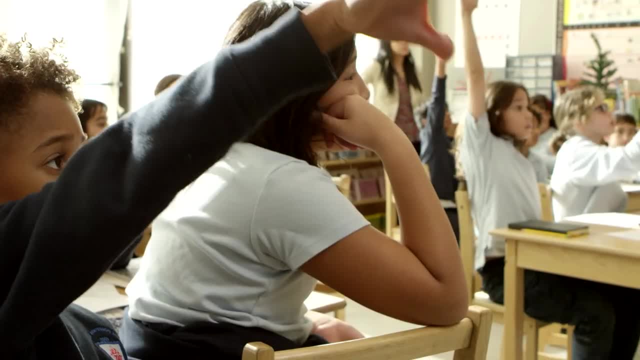 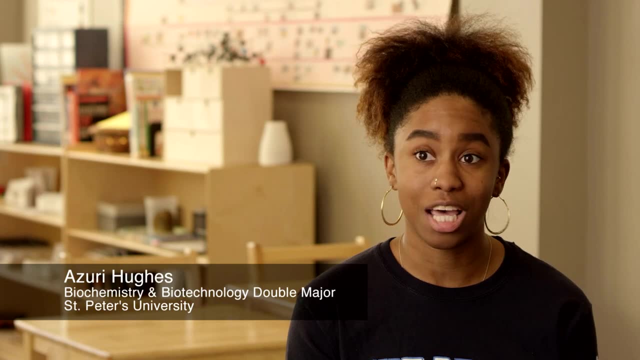 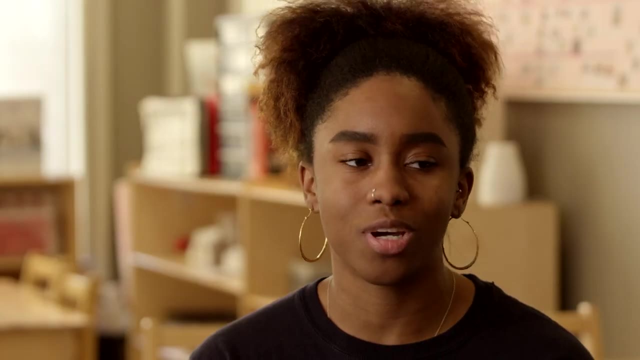 A whole semester to get these ideas. I remember when I was their age I never learned biochemistry at that level. What they're learning right now is really going to help them when they get to high school college. I really want them to be in the realm of STEM because they grasp it so easily. 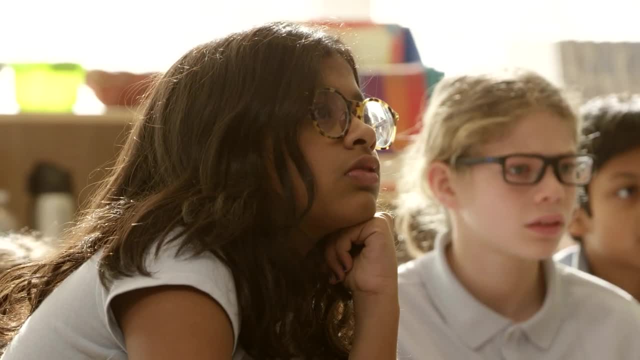 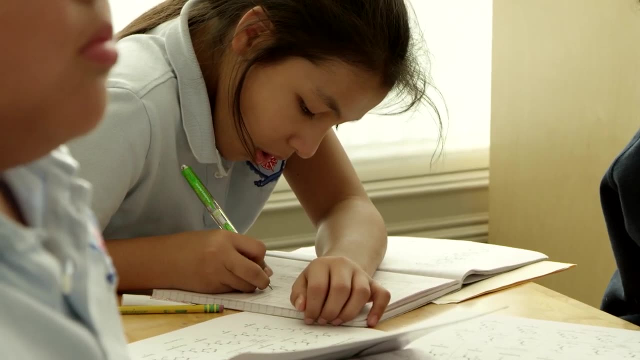 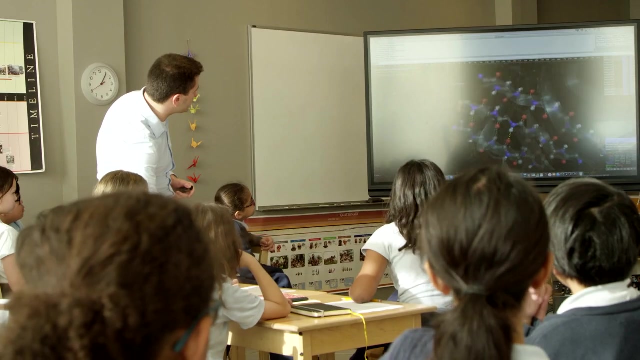 And you can tell that they are little scientists. So it makes me really happy- Me being a woman in STEM- and seeing other little girls learning biochemistry. Their curiosity sparked whenever there was a new concept on the screen. They were eager to ask me questions and they just wanted to know more. 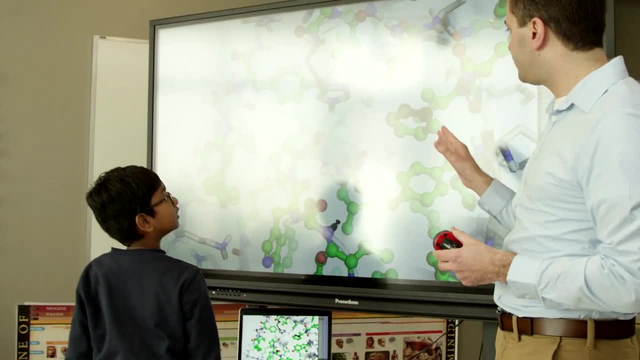 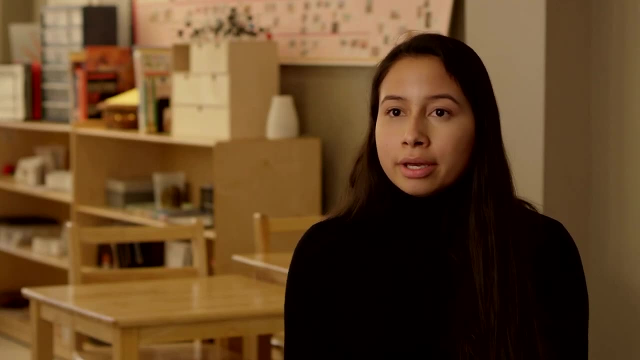 And these are things that college kids do not do. College students, they take this information for granted And they're given a new concept and they learn it. But in comparison, these kids, they want to learn how it's useful for them. 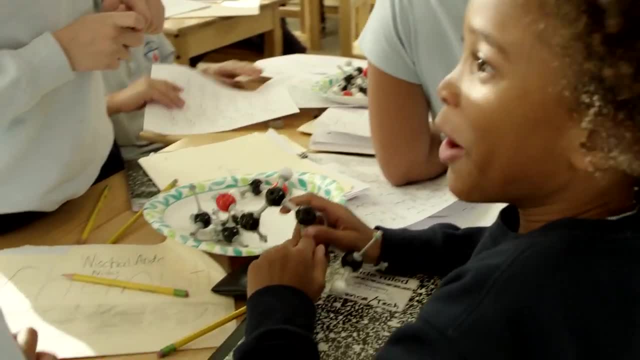 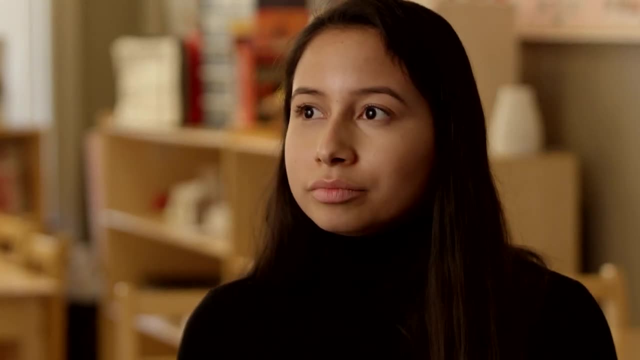 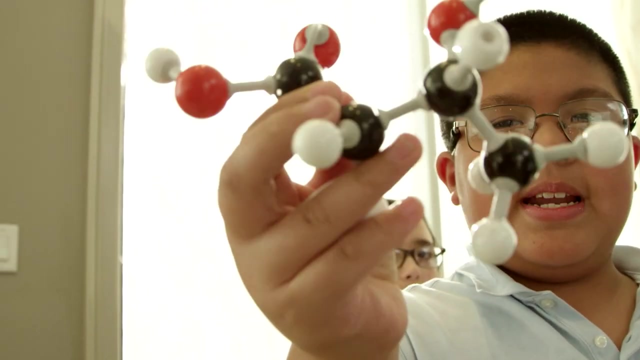 And whenever they were learning about amino acids, they wanted to know how many sulfur like is sulfur common in our bodies? And questions like that that most college students do not ask If I had the opportunity at their age to understand or experience science in this way. 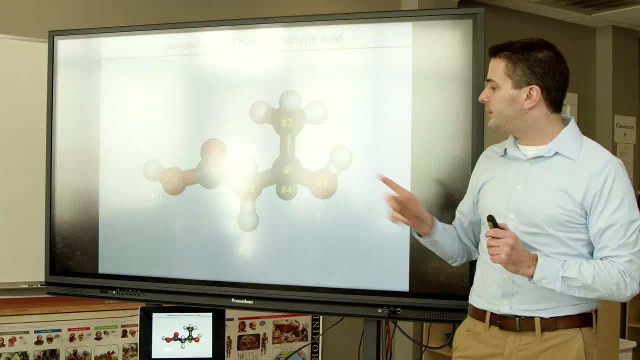 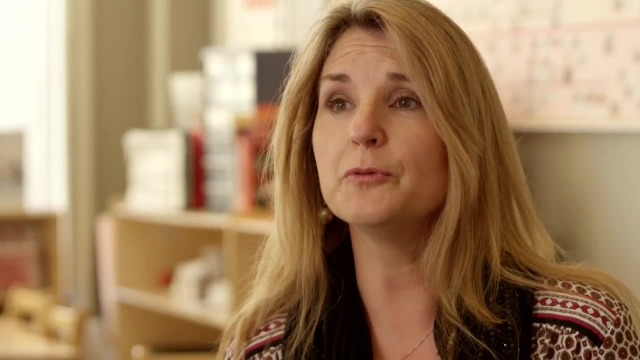 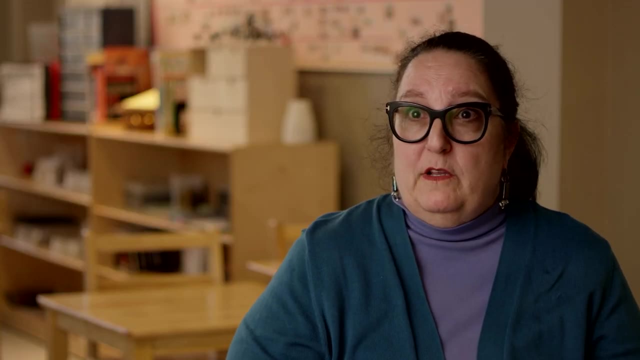 I think my life would have gone on a different track. He's allowing them to experience these ideas and these concepts without fear, without hesitation and just full of fun. Nobody ever says, oh do you remember that spelling test we took in second grade? 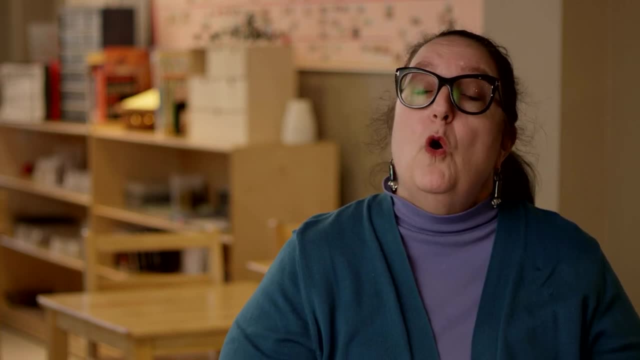 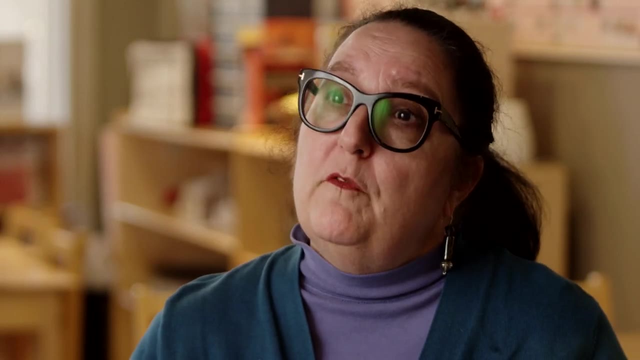 But they do say: remember that field trip that we took, Or remember that experience we had, And that is really a hallmark for young children. So if you provide these kinds of experiences, you're delivering something that most adults feel is important. It's way over their aptitude. 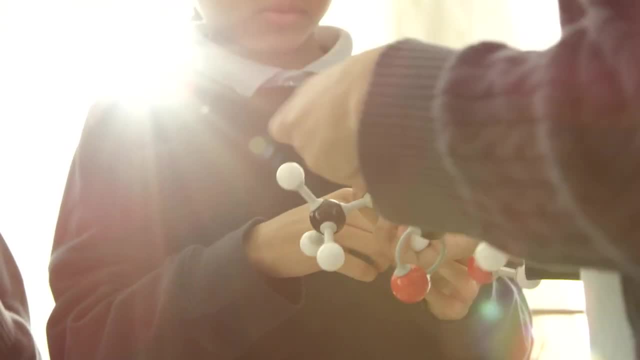 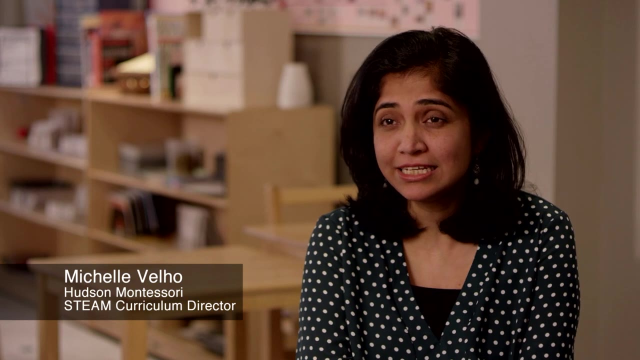 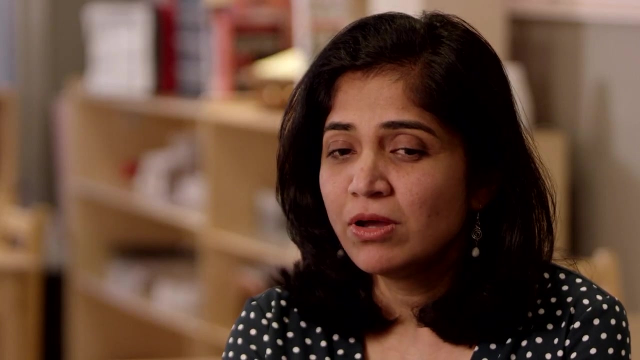 But in fact it is a real-life living experience for them. I'm really excited because I loved biochemistry as a child. It took me a while to understand how bonds are made and how molecules are made and how to balance equations, And so, even as a grown-up, I seem to be learning along with the children. 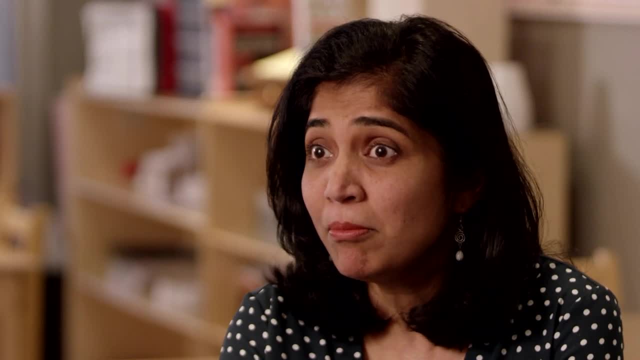 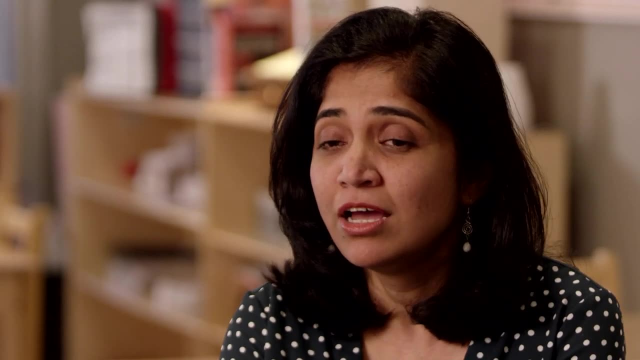 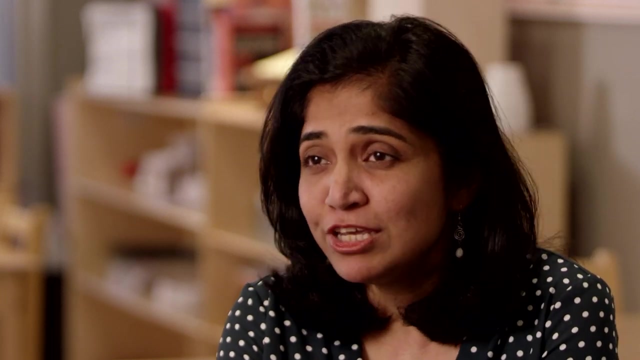 And then when I see things click for them at such a young age and get excited about the periodic table, and then suddenly they want to have a conversation about amino acids, they stop you in the hallway. So that excitement is something I feed on as an educator. 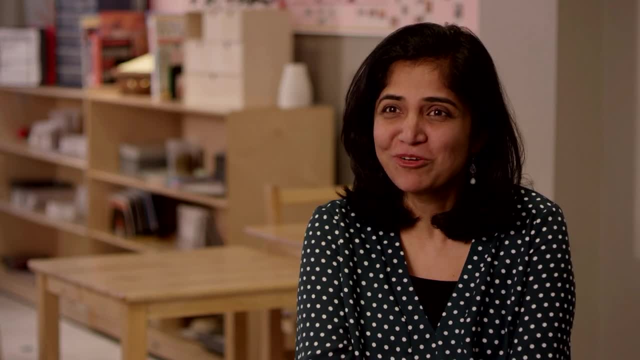 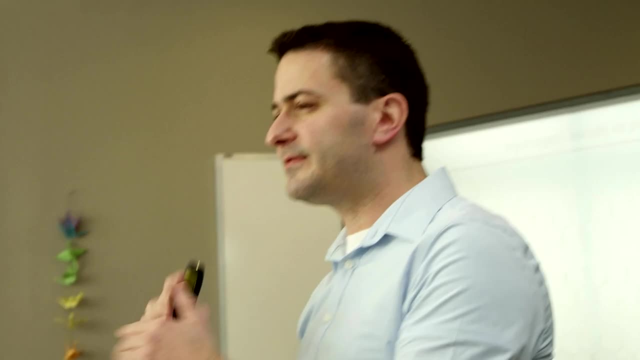 And suddenly biochemistry is now the next cool thing to do. Why do they have that specific amount of positive and negative charge? It has to do with this very stable configuration. So they're making more electrons to make pairs, so they can be like neon. 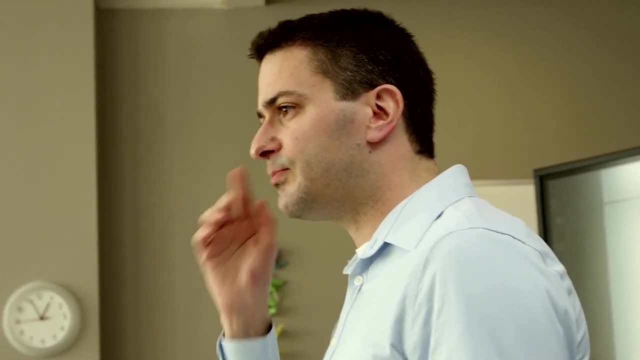 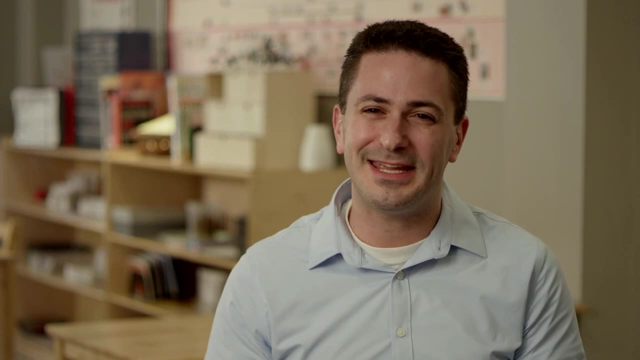 Yeah, exactly, They're trying to attain a noble gas configuration. That's what's driving so many things in chemistry: the drive towards a noble gas configuration. To get a competitive edge, students need many different kinds of educational resources, But what I feel like I'm doing here is not just giving them the content. 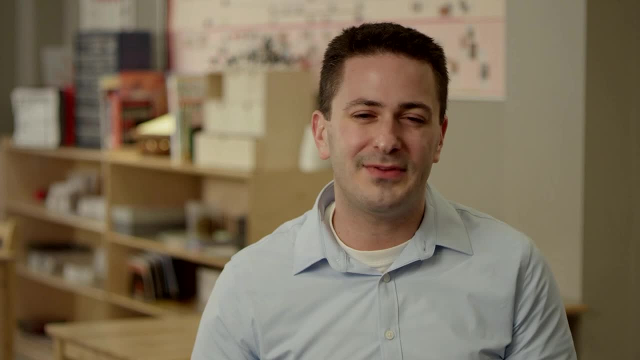 that they need to succeed in the future, but to also give them kind of an inborn passion about the subject, which students in other kinds of educational settings aren't going to get, that actually They may be learning similar advanced material at some point of their life. 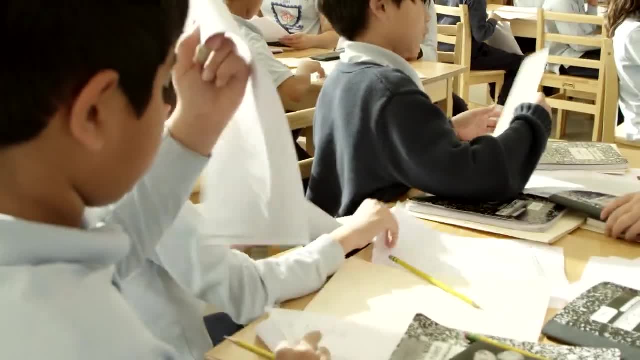 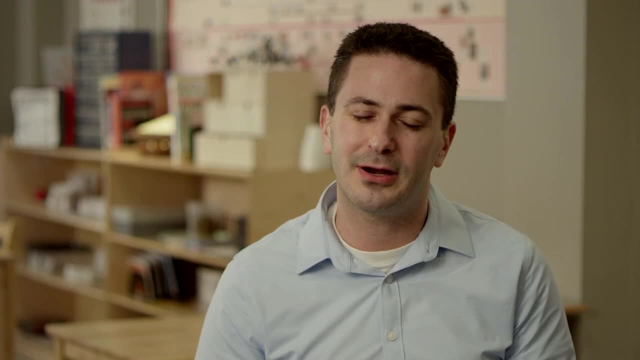 but what we're able to do here with the multidisciplinary approach is that we give them a self-directed drive to learn these subjects, and that's what can set students apart from the others that are maybe memorizing maybe, who are in it for the grade. 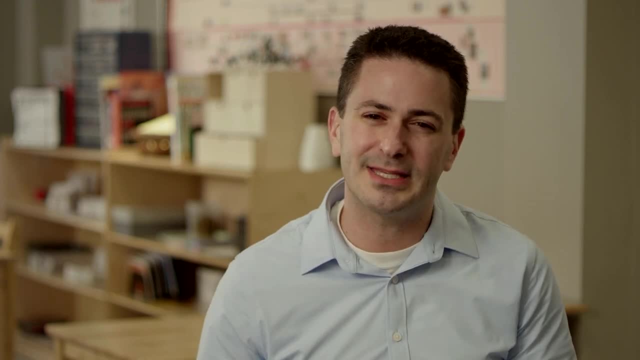 The kids that you see in these programs. they're not doing this for some grade. They're doing this because they have a passion and they see the importance of it and they see that they're learning also about themselves. they're learning what are they made of? 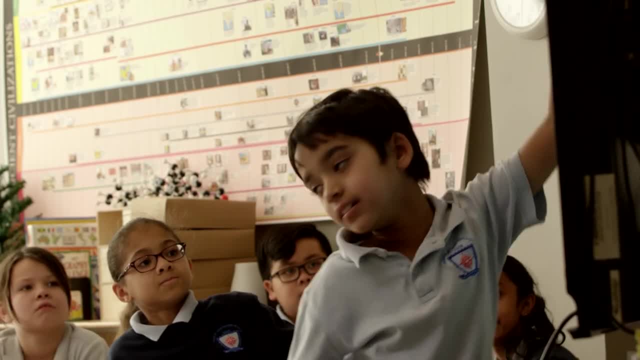 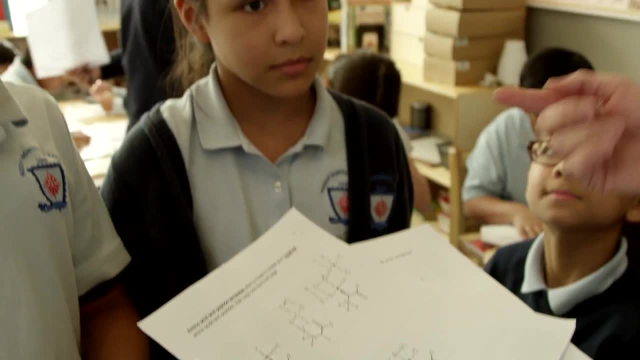 how are their senses connected to this amazing three-dimensional molecular world? So this one, she's got the charges right. She's got the base form of sulfur, which I didn't even teach that to you, so I don't know how you know that. 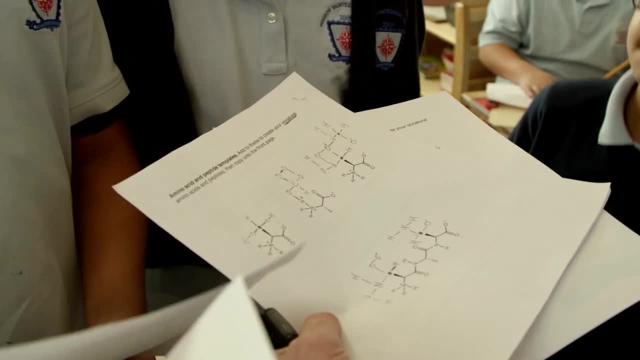 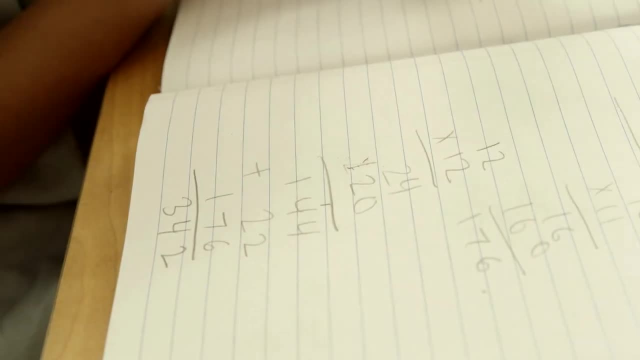 You have an interesting positive oxygen which is actually technically right. The bonding is really great. I mean, if you look at it, it's really mostly correct. So what's the answer? 342? Can you tell me So what? 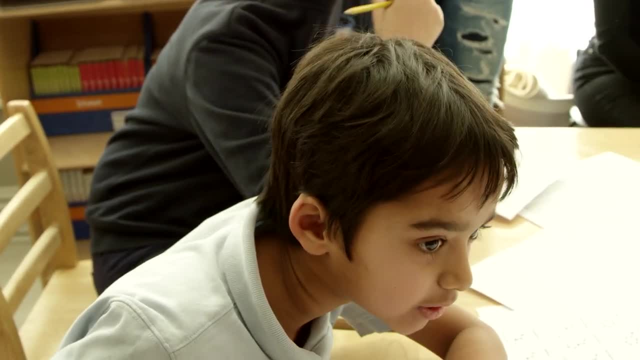 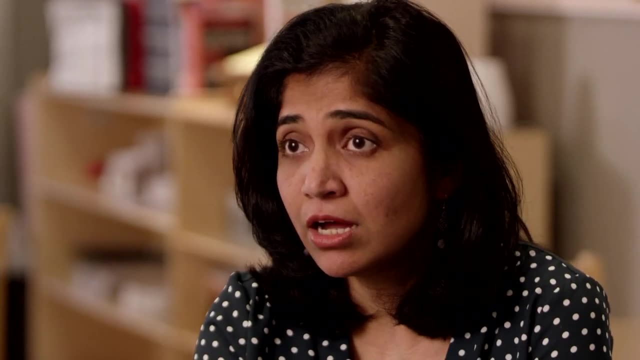 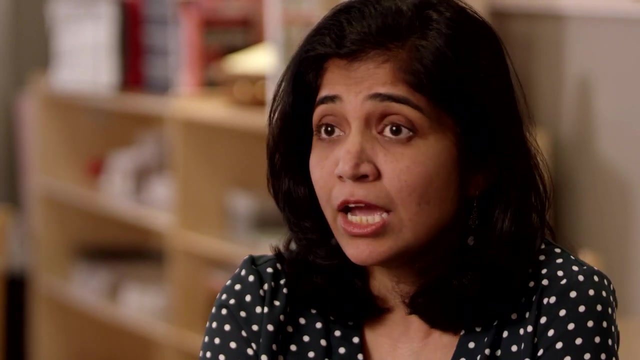 What is 342?? 342 is how much one mole of sucrose weighs: 342 grams. This foundation that they got with biochemistry allowed me to explore chemistry with the other topics like air quality or water pollution or even plastic. Why is plastic taking so long to biodegrade? 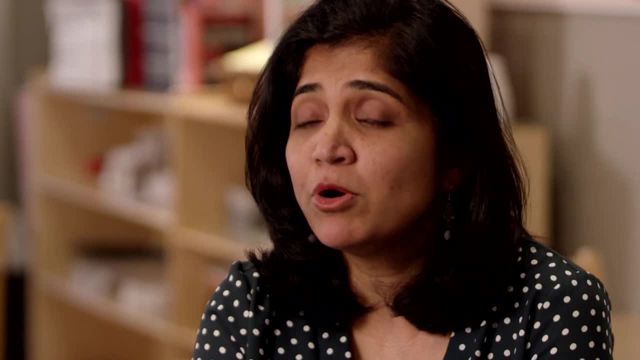 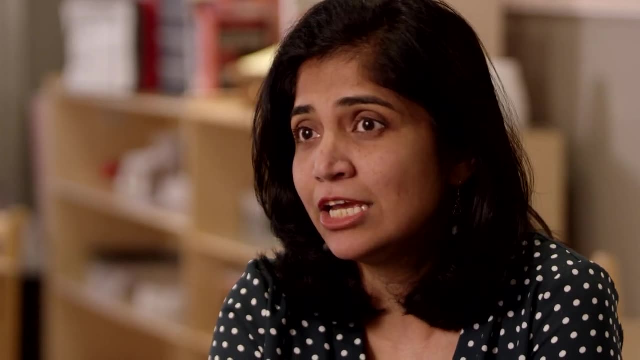 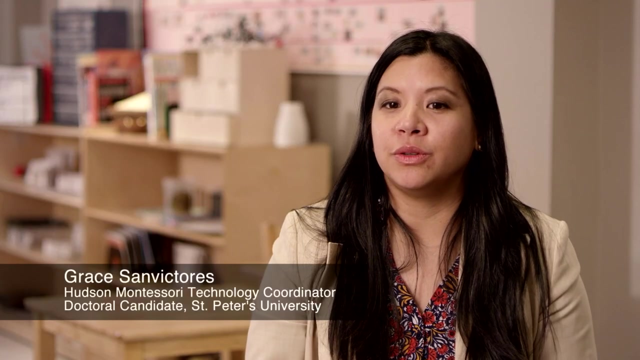 Is it something in its molecular structure? So I can pose these questions now to my students because I know they have that basic foundation and understanding. There's many moments where we are doing our own curriculum and they go back and refer to Dr Fried's lesson. 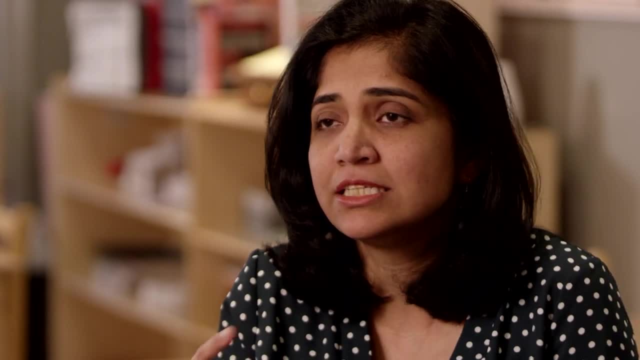 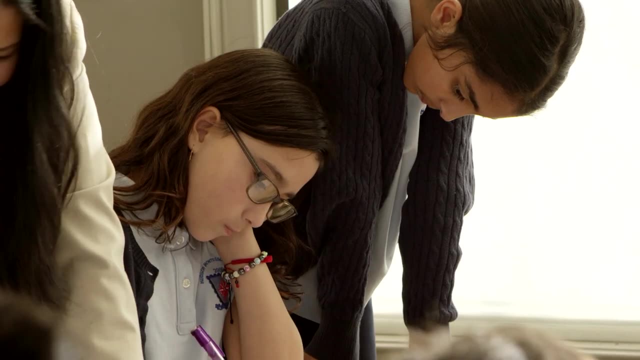 I can take it with a chemistry lesson, I can take it with a physics lesson, I can take it with a biology lesson. It's easy for me to make those connections with whatever topic I'm trying to do. In fact it has led many of my 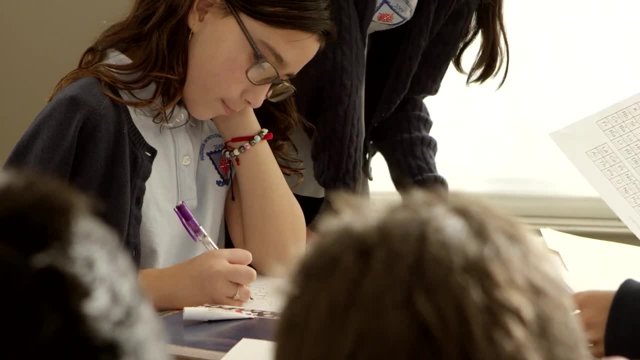 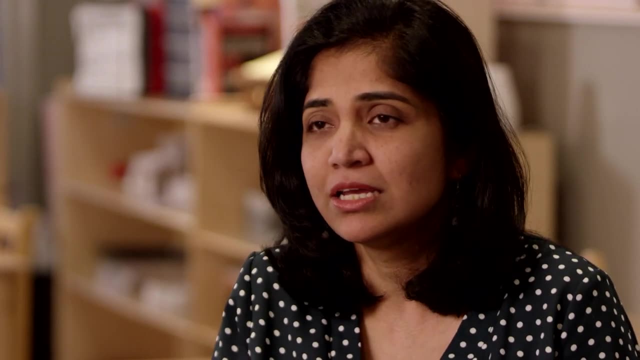 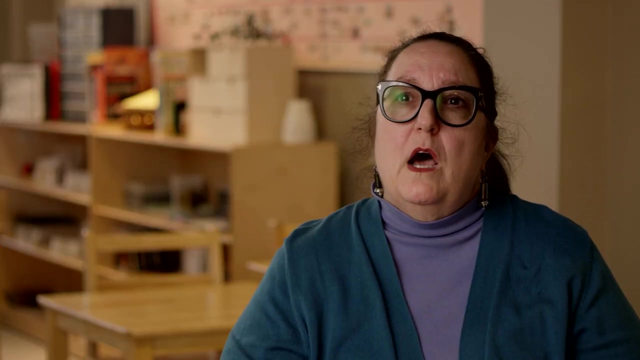 follow-up lessons and experiments, because we can always go back and say: remember what you studied in Dr Fried's class. So any concept that I'm talking about comes back to the fundamental unit of matter, which is atoms. I would also say that we're not all. 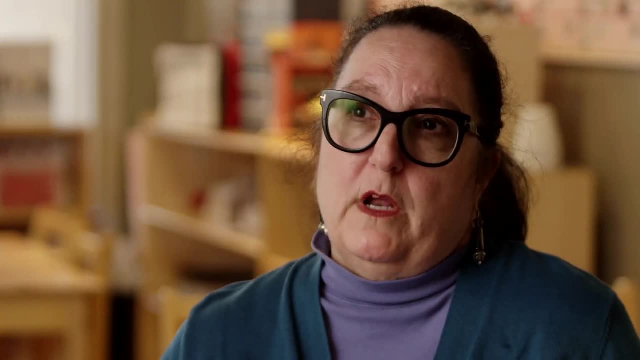 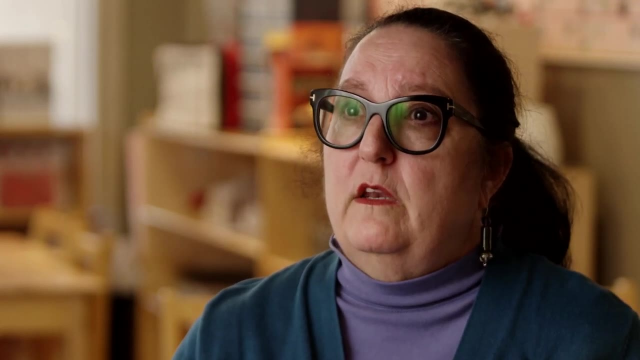 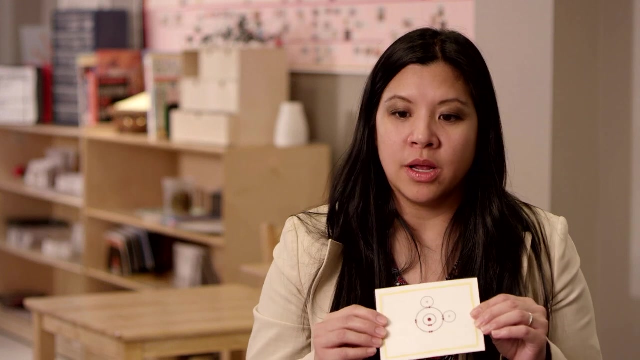 cookie-cutter kinds of learners. Some of us are predominantly an auditory learner, Some of us are more predominantly a visual learner And some of us need more of the kinesthetic and tactile kinds of things to help us along. Our approach to learning is to meet all their sensory. 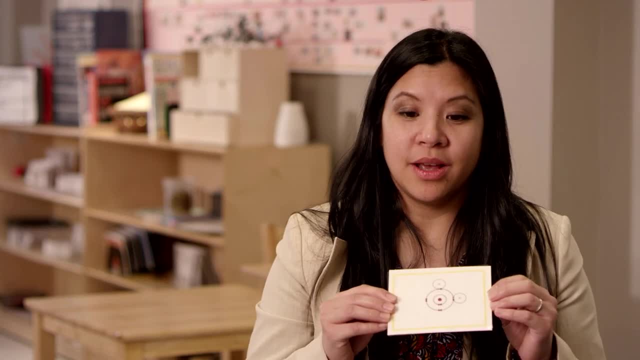 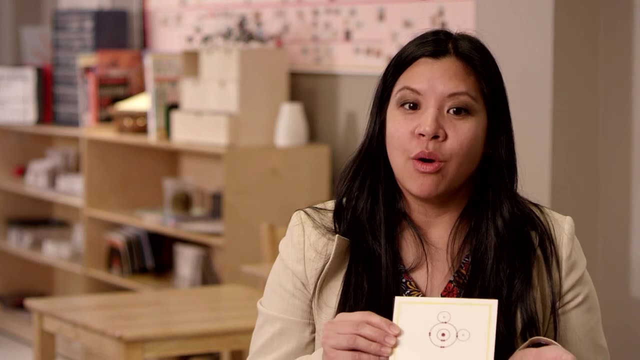 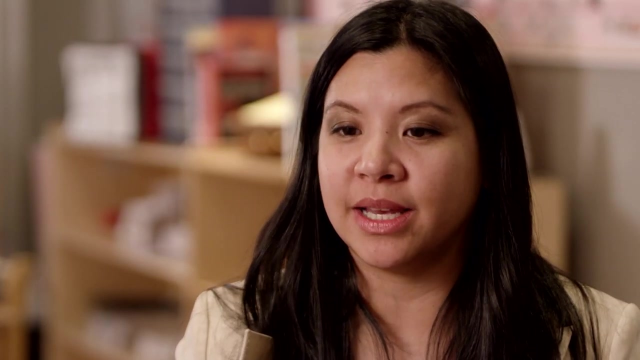 Sense of touch, sense of sight, sense of smell. He's presented lessons where he's brought in vinegar and oil and they smell that, but they can also see why water doesn't mix with oil And so it's a simple experiment, but he connects it. 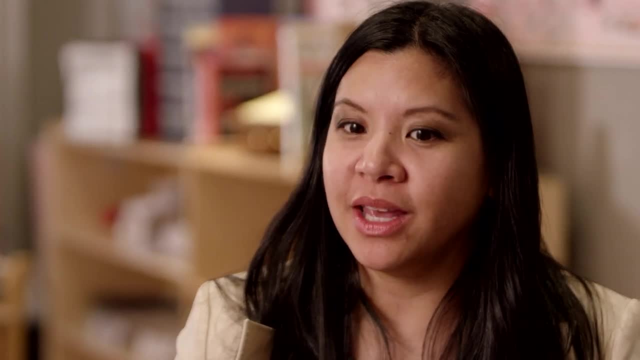 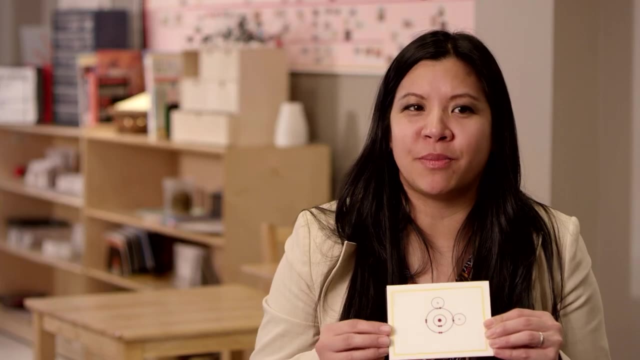 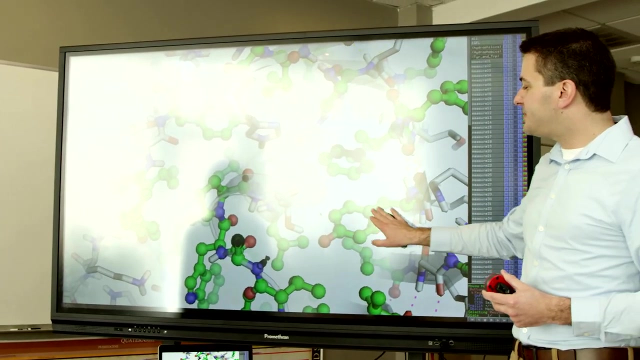 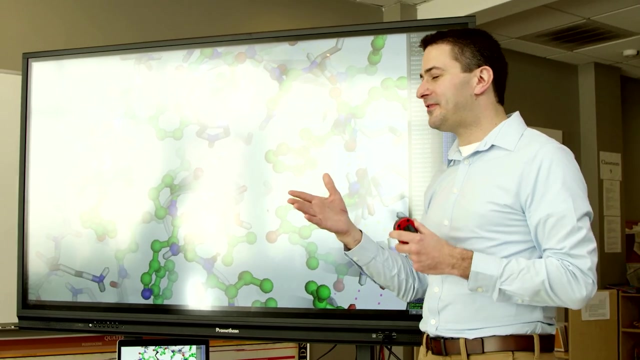 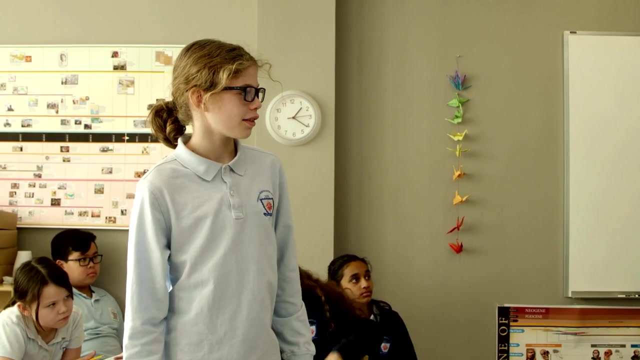 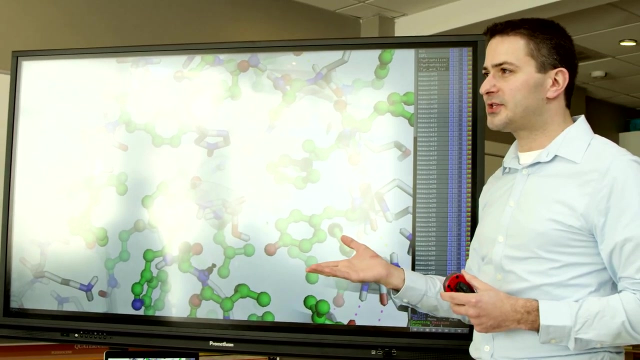 with how bonding works and they could see. oh, that's why, because it's hydrophobic or hydrophilic- And you see them using these words that you wouldn't expect a fourth grader to say- One of the things we appreciate with Dr Freed's. 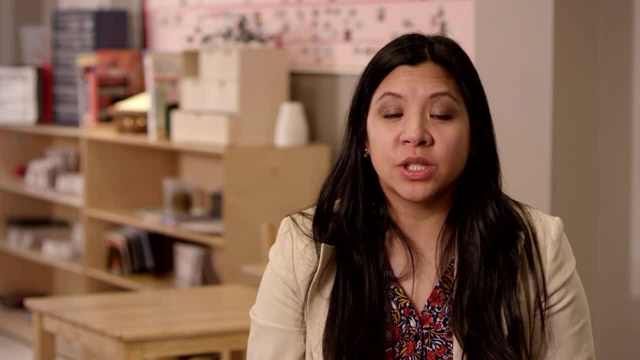 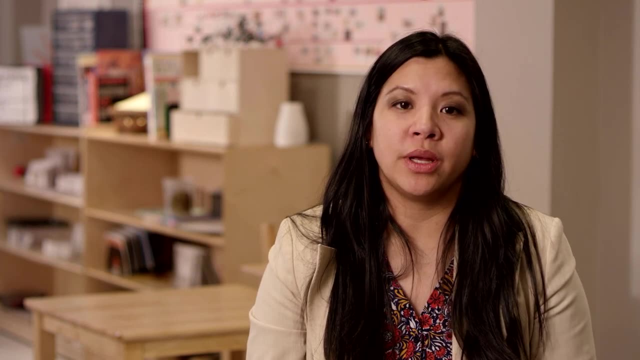 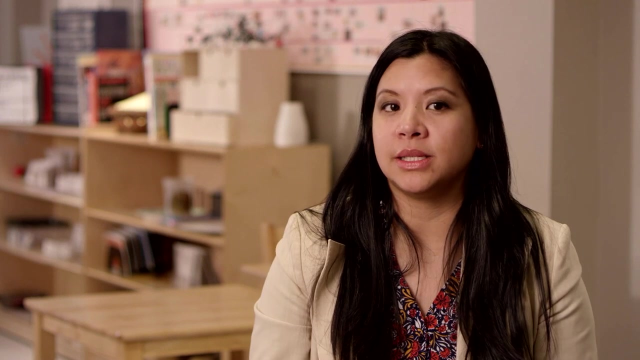 program is. he was able to actually personalize his program with our school. We've talked to him about our methodology, and Montessorians use certain tools as well, and so he's customized his lessons so that it complements our lessons as well. For example, we have this: 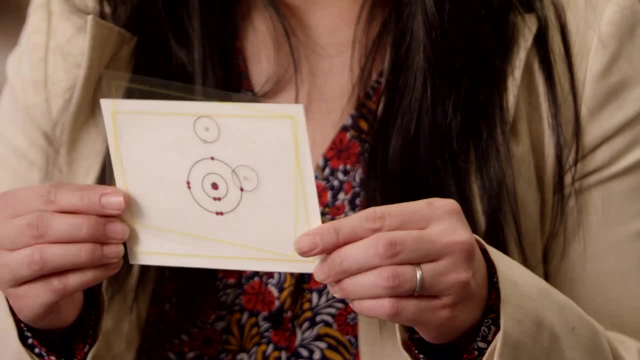 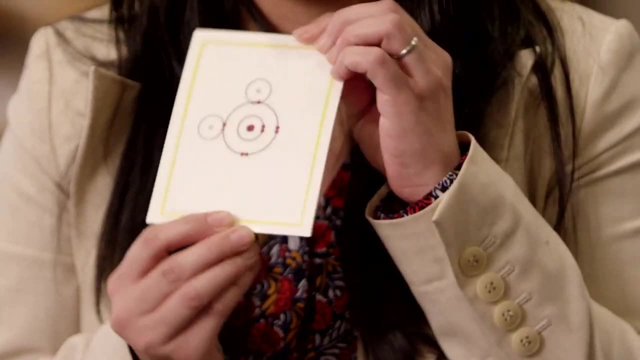 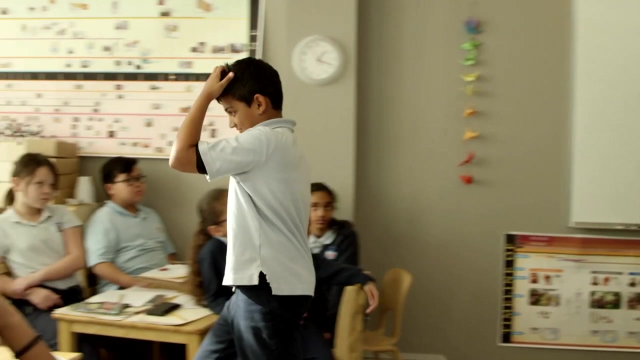 card and it's transparency, and it shows bonding and how electrons look for pairs, and so we come up with this Mickey Mouse molecule that we call water. Our goal here is to equip them with 21st century skills and with Dr Freed's program that allows them to. 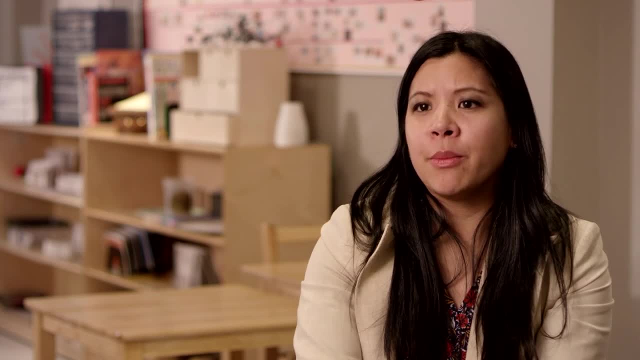 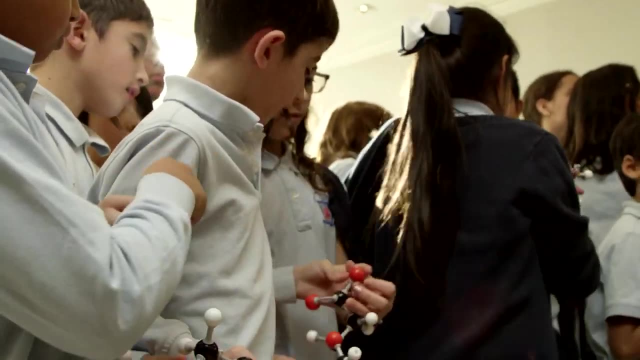 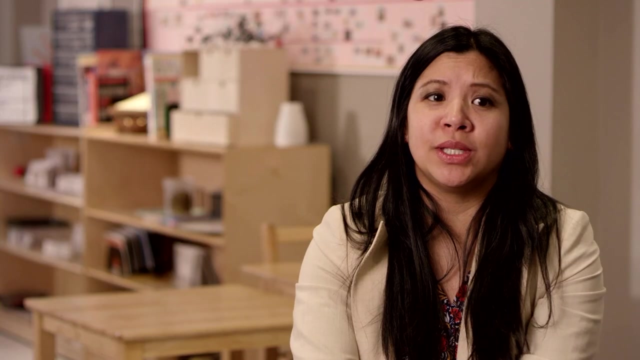 obtain those soft skills such as collaborating teamwork. they're building polymers and peptides together and talking it out with each other. I mean, the room does get loud but you see them engage and they're excited and they want to learn more. When he introduced 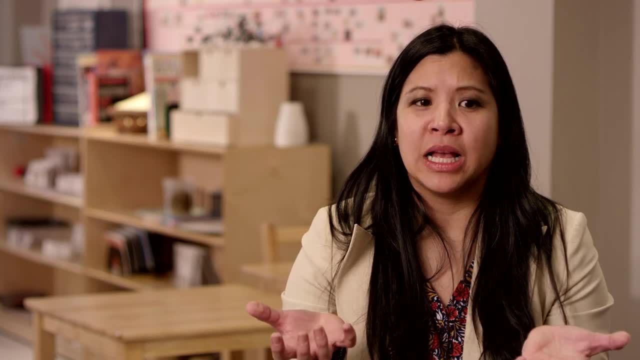 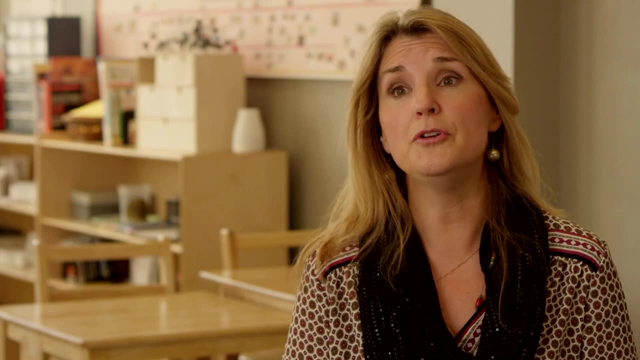 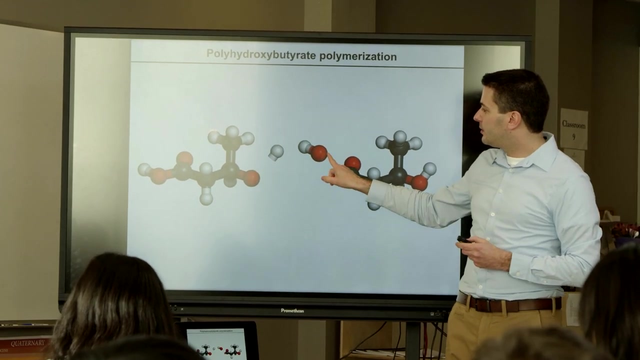 biodegradable plastic and they're holding the molecule and they're like. so this is that, and that, for them, is mind blowing. This is a program that would benefit all students, not just a select few. The benefits that we're seeing with our children. 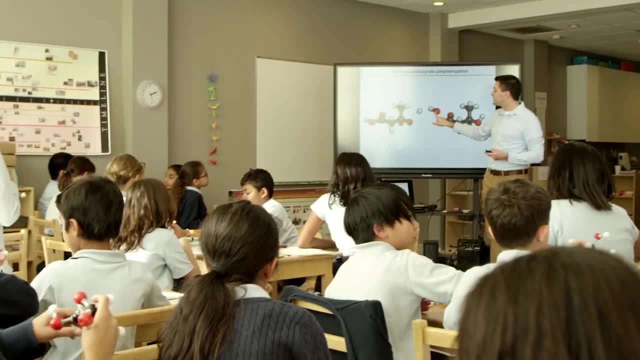 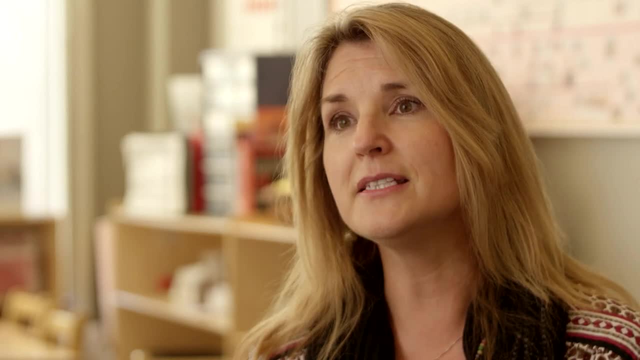 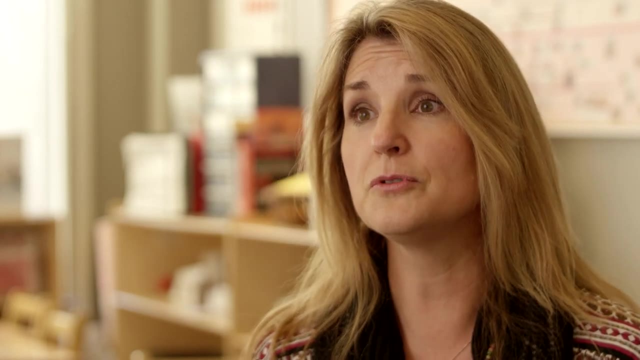 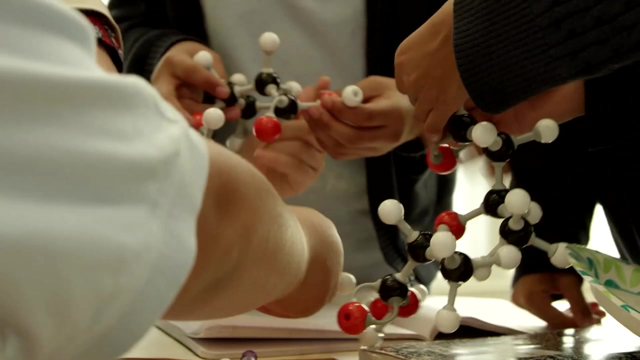 go far beyond and after the class ends, They are applying it in their everyday lives. They are showing that this is something that holds great value and it deserves to be used by all students. And we need more sciences, especially in research. There's so much research that can be. 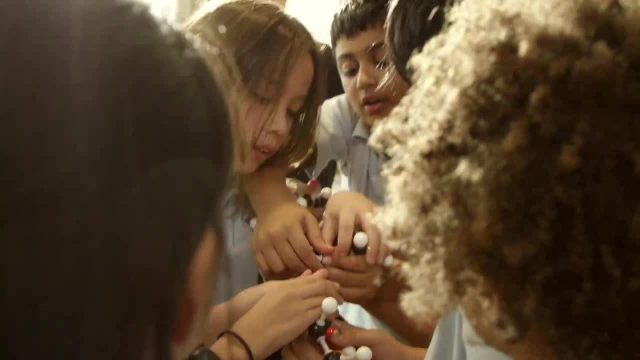 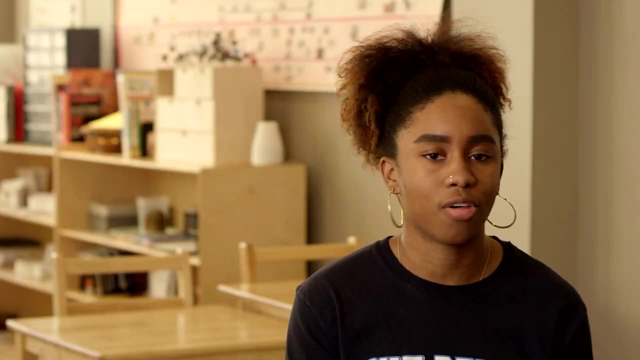 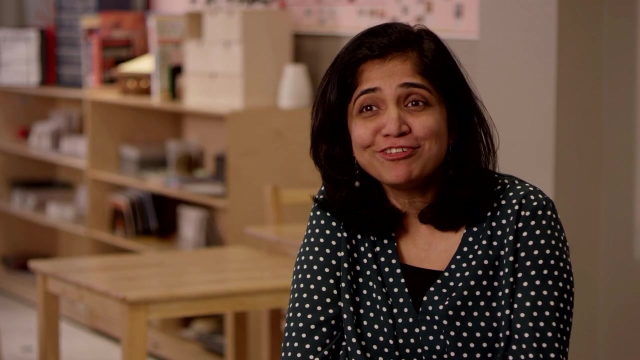 done on everything in terms of developing advancing health, healthcare, biotechnology, cancer, all of that. It's not just elementary elements, It's more than that. Personally, I am now more confident to talk biochemistry, even though I majored in it, Having sat in on 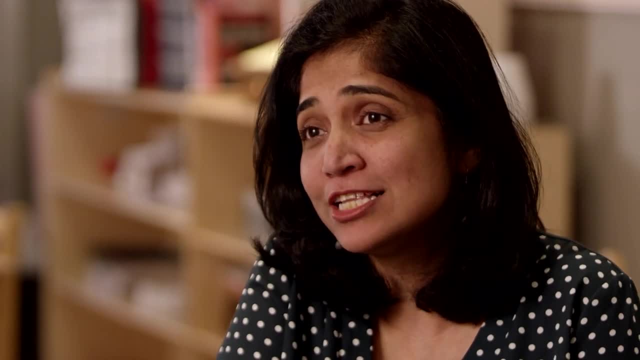 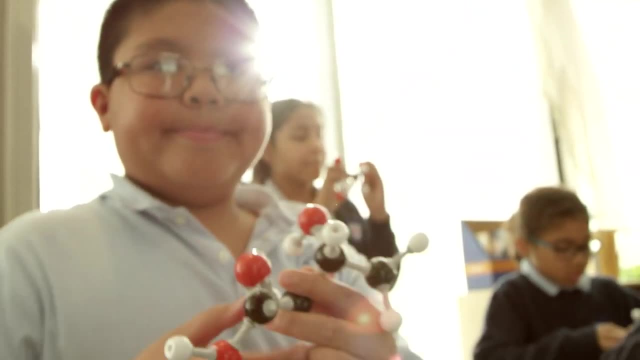 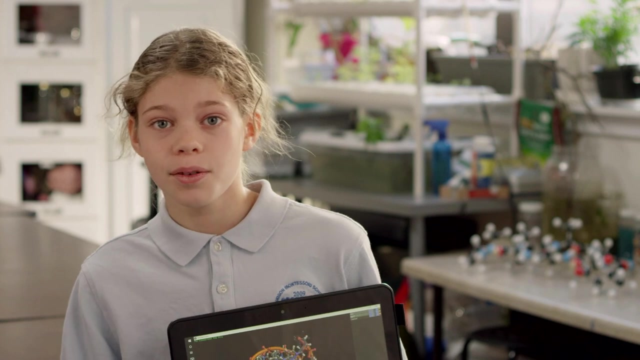 Dr Freed's class, I am more confident of teaching these concepts to children, and if they're curious and excited to learn about something, then let's give them more In the future. I would like to learn how cells are made by molecules, because there's DNA in cells. 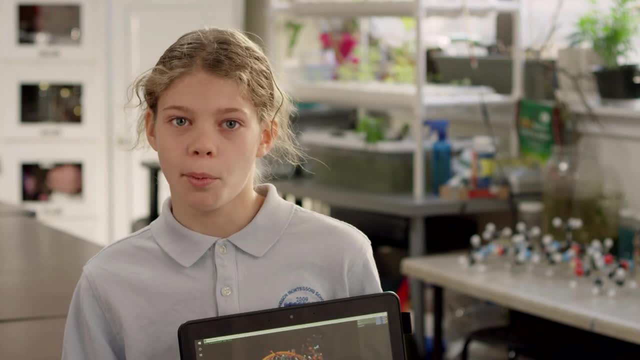 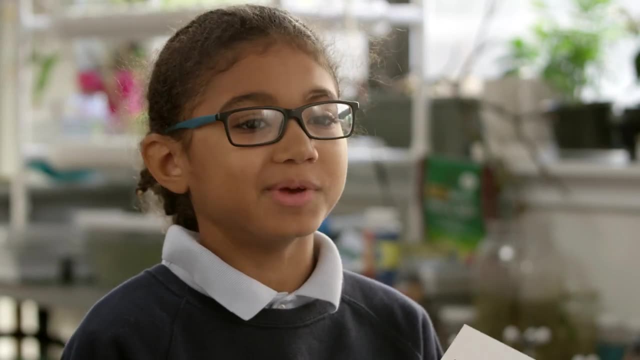 nucleus, and there's way more in cells that I don't know about, so I want to know about it. Well, I feel like, since I know this, I'll be a great student in college and I'll know I'll be an extra step ahead of everyone else. 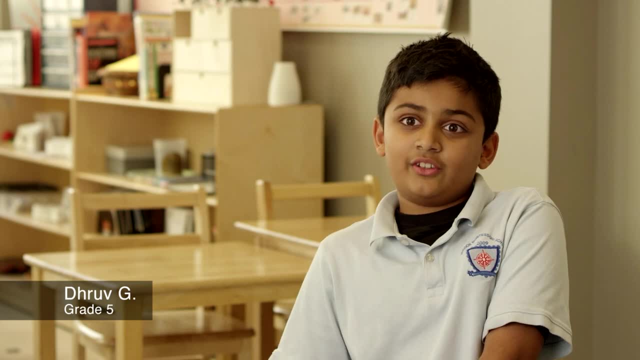 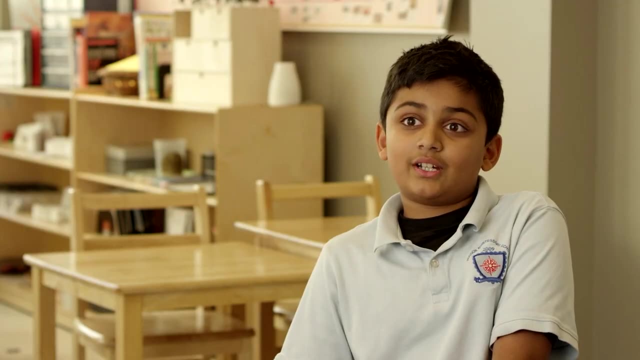 Part of the Montessori program is to go to the United Nations to speak. Now I'm very confident to speak in front of 2,000 people about climate change and I'm mentioning the problem of CO2, carbon dioxide- and I learned about it.